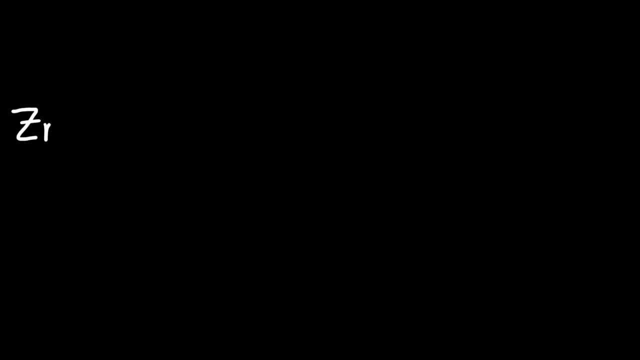 Here's a question for you. Let's say we're reacting zinc metal with aqueous copper chloride. Will the reaction proceed, or should we write no reaction? How do we tell? How do we find the answer to that question? Now there's something called the activity series which can help you. 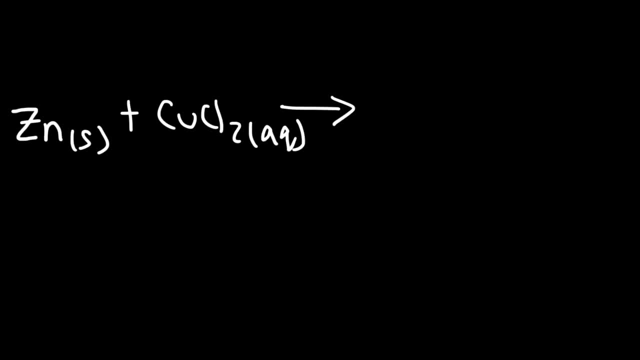 to determine if a reaction will proceed or not in a single displacement reaction, which is what we have here Now. you can look up the activity series in Google Images if you want a complete list, but I'm just going to give you some of the elements just so you can answer the questions. 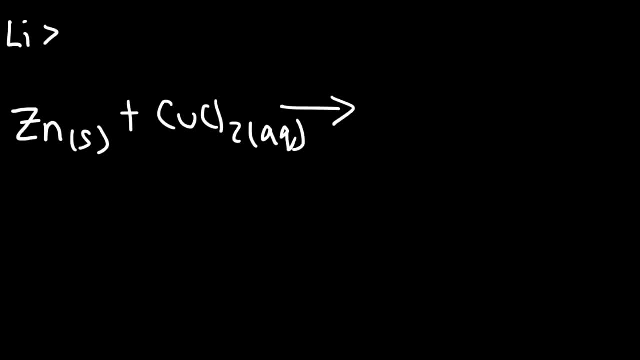 in this video. Now you need to know that lithium is more reactive than sodium, which is more reactive than magnesium. and then you have aluminum, zinc, iron, metal nickel, hydrogen and sodium. Now you have copper, silver and gold. Silver and gold are the least reactive noble metals, so make 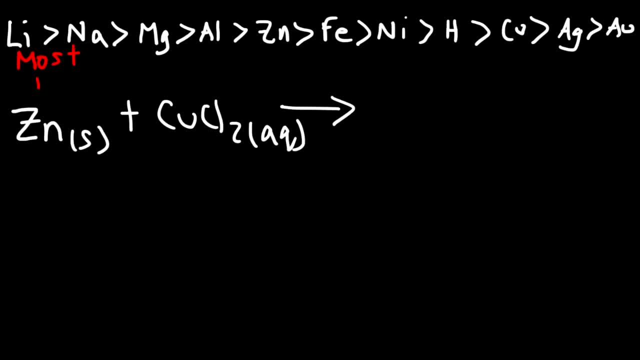 sure you understand that lithium is the most reactive, and so reactivity increases towards the left And elements like silver and gold. they are the least reactive. So now let's go back to the question that we're dealing with. How can we determine if there's going to be a reaction? How can we use the activity series to find the answer? 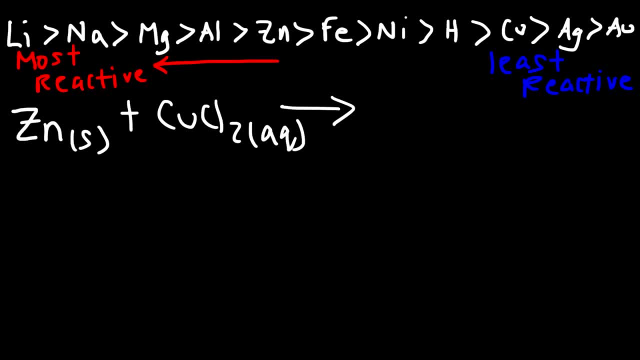 You need to ask yourself a question: Can solid zinc metal displace the copper in the aqueous solution? Is zinc metal stronger than copper? And so, looking at what we have, zinc is to the left of copper, And so we can say that zinc is stronger than copper. 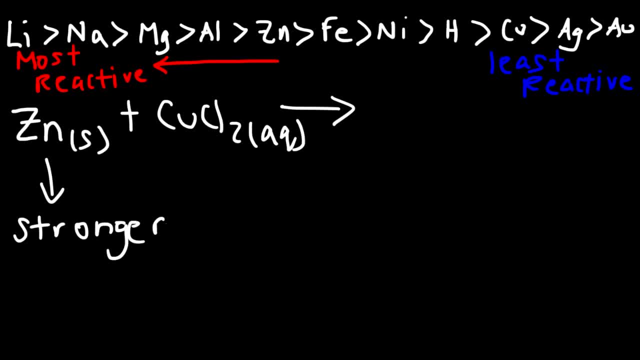 So the reaction will proceed. So now that we know that the reaction will work, how can we determine the products of the reaction? So this is a single displacement reaction. We have element A reacting with a compound which we could say compound BC. 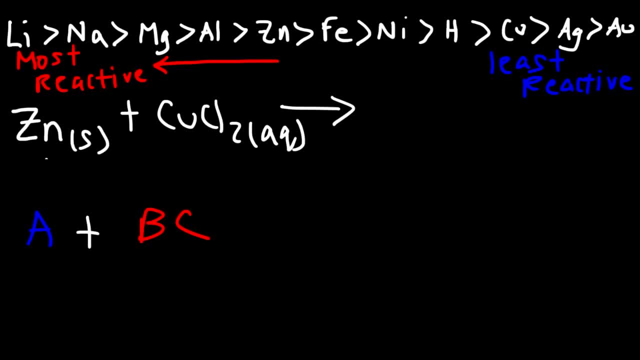 A is zinc, B is copper, C is chlorine, And so what's going to happen is A is going to kick out B and pair up with C, So B is going to be by itself and A will be attached to C, So in this case, copper will be by itself. 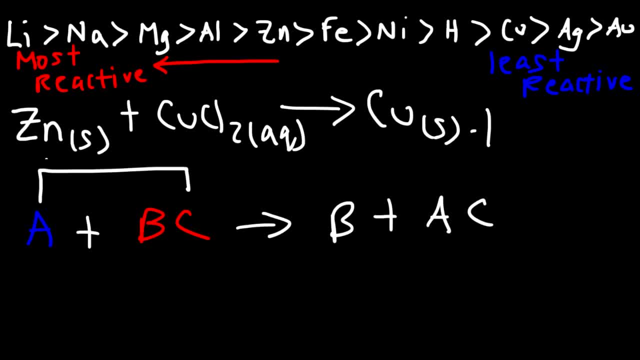 It's going to precipitate out of the solution as a solid And zinc is going to pair up with chlorine. Now, whenever you're writing an ionic compound, you need to make sure that the charges are balanced So that you can write the formula correctly. 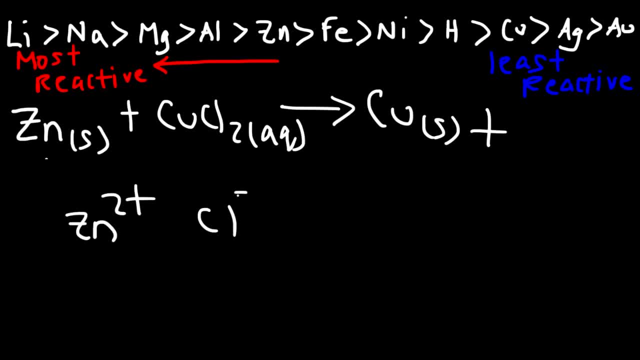 Zinc as an ion has a 2 plus charge. Chlorine has a minus 1 charge. So to balance the charges we need two chloride ions to pair up with the zinc 2 plus ion. So the formula is going to be ZnCl2.. 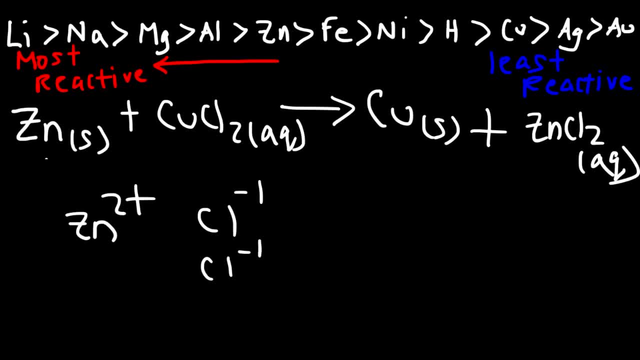 And because it's soluble in water, we're going to write Aq. It's going to dissolve in water. It's going to be in the aqueous phase. Now, let's try this. Let's try another example for the sake of practice. 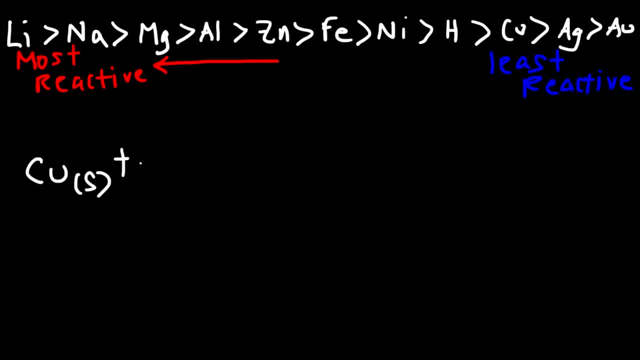 Let's react copper metal with iron 2 sulfate. Go ahead and try this problem, So using the activity series. will this reaction proceed? as written? Will it work? Is copper strong enough to displace iron out of the solution? Now copper is to the right of iron metal. 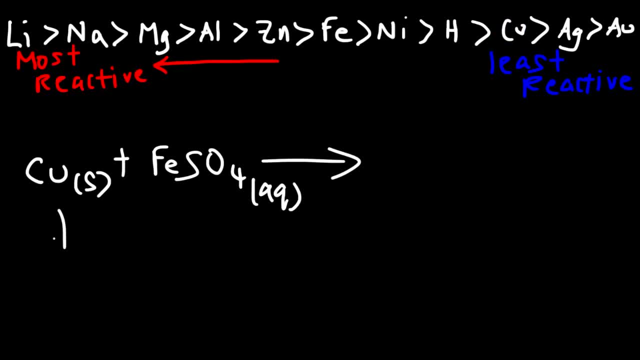 So therefore we could say that copper is weaker than iron metal. So because it's weaker, it cannot displace iron metal out of the solution. So for this example, there's going to be no reaction. It will not work. Copper is less reactive than iron metal. 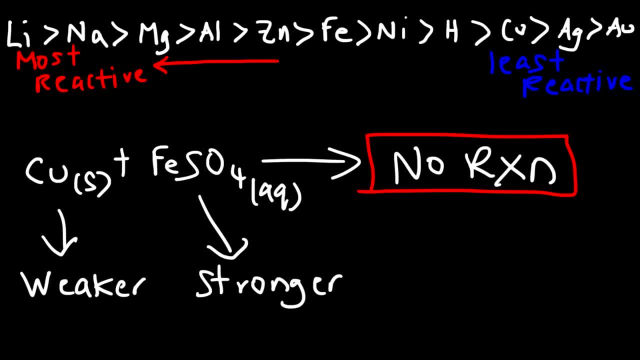 And so that's how you can use the activity series to determine if a single replacement reaction will proceed as written or if there's going to be no reaction. Here's another example: Let's make solid Aluminum metal with aqueous hydrochloric acid. 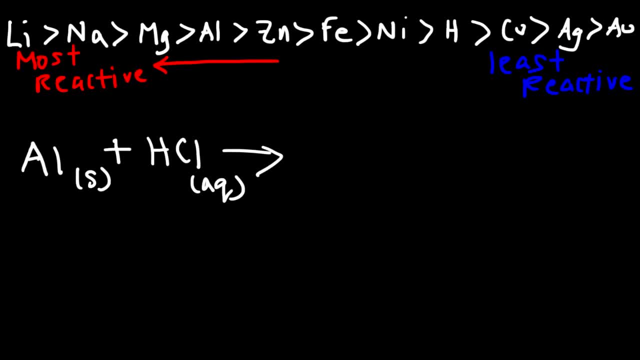 Will the reaction proceed as written? So using the activity series, what would you say? Is it going to work? or should we write no reaction? Is aluminum metal? is it strong enough to displace hydrogen out of the solution? So, aluminum metal, is it strong enough to displace hydrogen out of the solution? 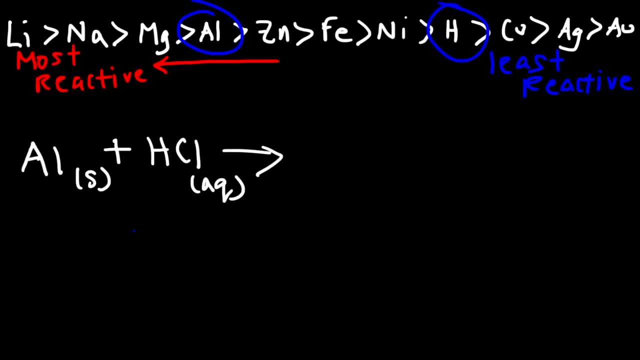 Aluminum metal is to the left of hydrogen, so it's more reactive. So we could say that aluminum is stronger in terms of chemical reactivity relative to hydrogen. So, yes, this will work. So aluminum is going to displace hydrogen, And so we're going to write it as a pure element. 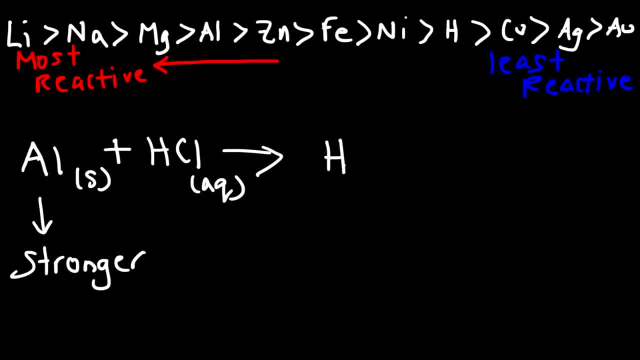 Now hydrogen. you don't want to write just H. It's a diatomic gas, So you need to write H2.. And then aluminum is going to pair up with the chlorine. Now aluminum has a 3 plus charge as an ion. 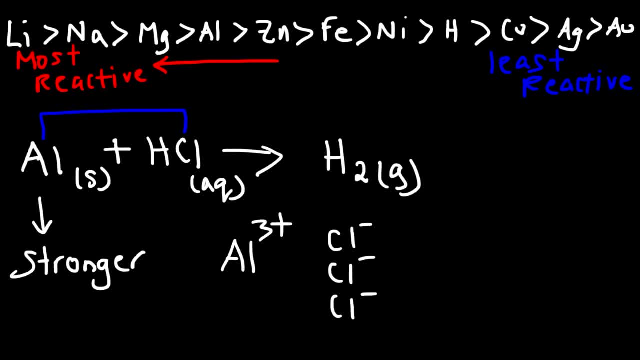 So we need 3 chloride ions to balance the positive 3 charge on the aluminum cation. So to write the formula, it's going to be AlCl3.. And it's soluble, so we're going to write Aq. So that's how you can predict the product. 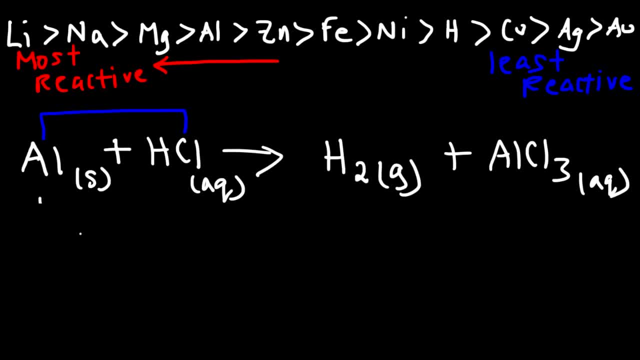 So that's how you can predict the products of a single replacement reaction. Now the next thing that we need to do is balance the chemical equation. So what coefficients can we write such that all of the atoms in this equation will be balanced? So right now we have 3 chlorine atoms on the right side, but only 1 on the left side. 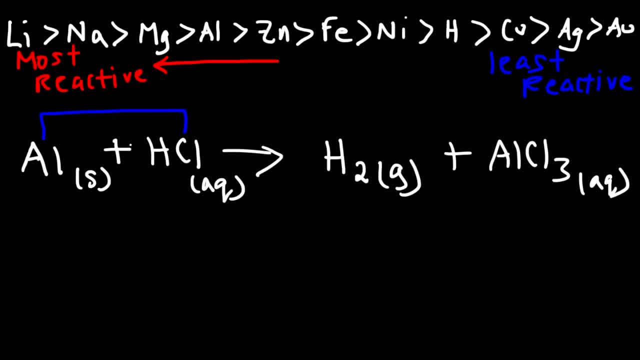 So that may indicate that we need to put a 3 in front of HCl. Let me use a different color Now. if we do that, the number of hydrogen atoms will not be balanced, And to make it equal, we have 3 hydrogen atoms on the left. 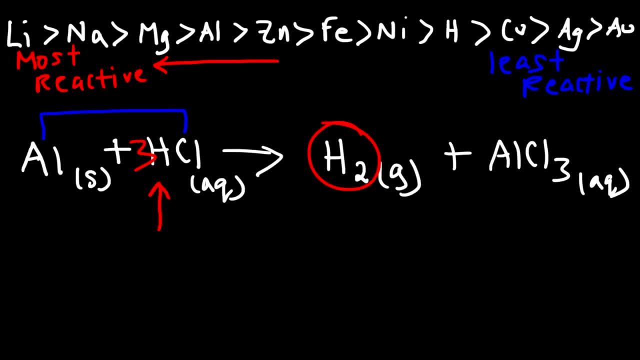 Right now we only have 2 on the right. So what do you think we need to do To make it equal? we need to use a fraction 3 over 2.. Because 3 over 2 times 2, the 2's will cancel and you'll get 3.. 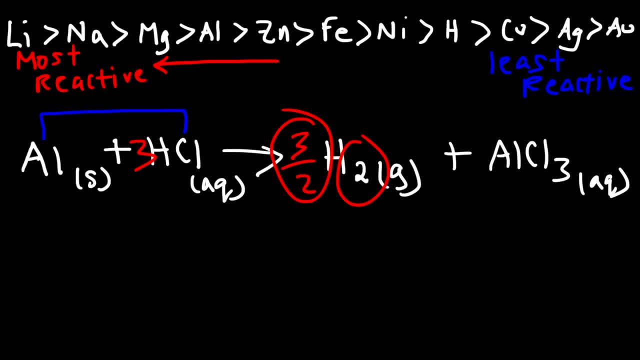 However, we don't want to deal with fractions when writing the coefficients of a balanced equation. We want to use whole numbers, And so what I'm going to do now is I'm going to double everything. So I'm going to start by putting a 6 in front of HCl. 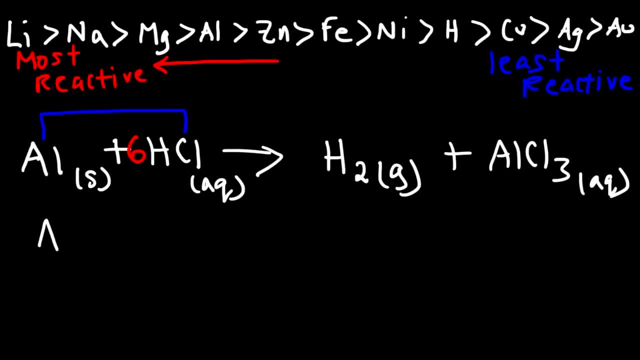 So now I have 6 hydrogen atoms. If you want to write it out, you can do it this way. So I currently have 6 hydrogen atoms on the left side, 1 aluminum atom on the left and 6 chlorine atoms. 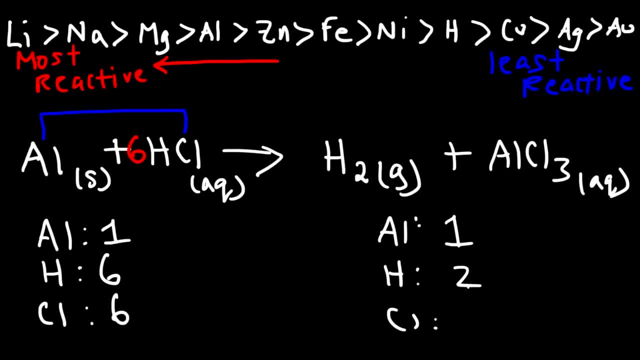 On the right side, I have 1 aluminum atom, 2 hydrogen atoms and 3 chlorine atoms. So I need to put a 3 in front of HCl And I'm going to put a 3 in front of H2, such that I will now have 6 hydrogen atoms on both sides. 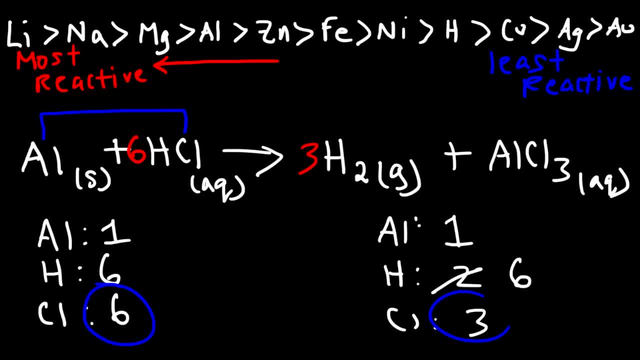 Now the next thing I need to do is balance the chlorine atoms. I have 6 on the left, 2 on- I mean 3 on the right, rather. So what I need to do is put a 2 in front of AlCl3.. 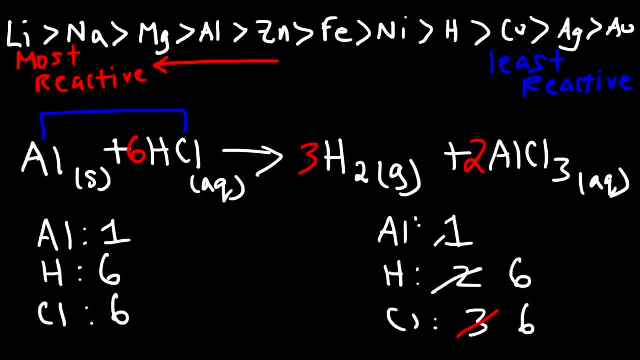 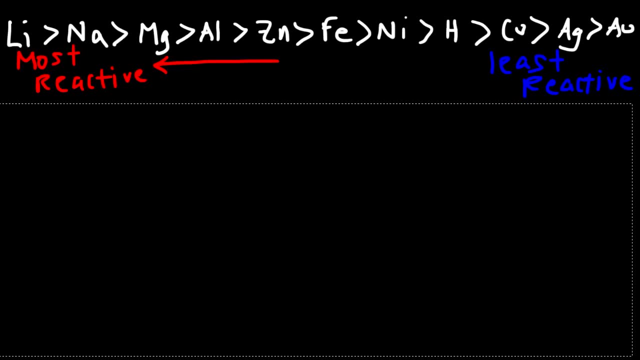 So this will now become 6. And this changes to 2, so I need to put a 2 in front of Al, And now everything is balanced, And so that's it for that example. Now let's talk about writing chemical reactions with halogens as it relates to single displacement reactions. 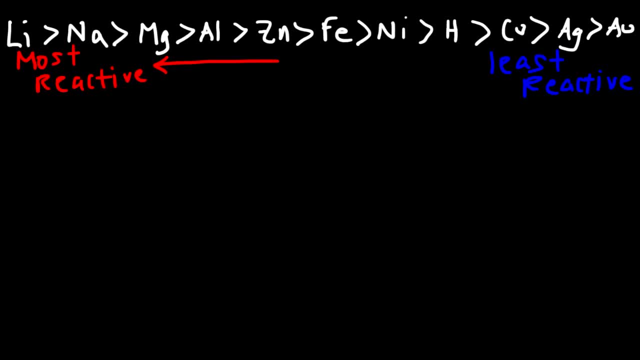 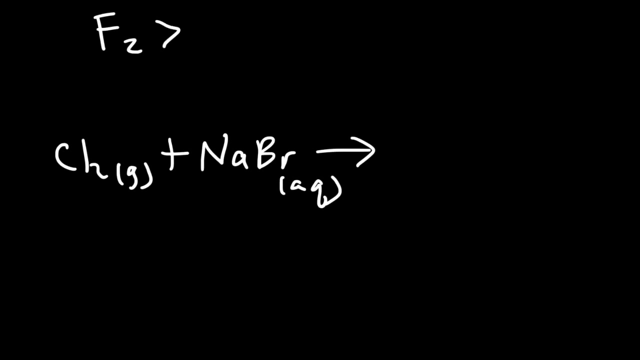 So let's say, if I'm reacting chlorine gas with aqueous sodium bromide Or aqueous sodium bromide gas with aqueous sodium, With the reaction, proceed as written. what would you say? Well, let's find out. For the halogens you need to use a different activity series. You need to know that fluorine is the most reactive halogen. It's more reactive than chlorine, which is more reactive than bromine, And that's more reactive than iodine. So how does it matter? But I do not have a that solution. 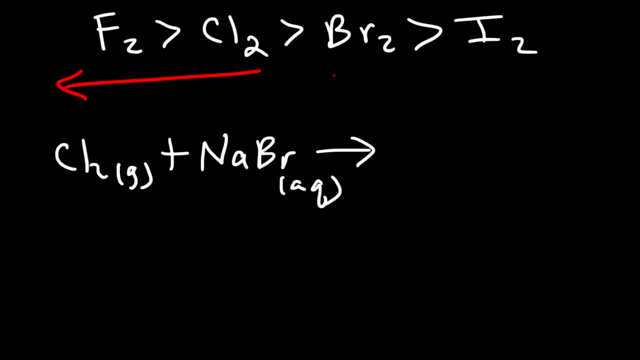 so reactivity increases to the left. so using that particular activity series, can we say that chlorine is strong enough to displace the bromide ion out of the solution? a halogen will displace another halogen out of the solution if it's strong enough, but in previous examples we considered a metal. 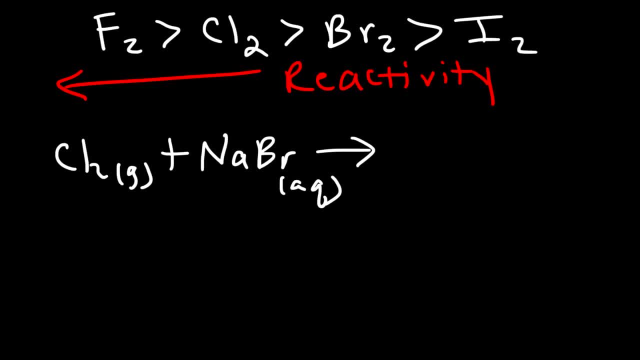 displacing another metal out of the solution, with the exception of hydrogen, of course. so using this activity series, we can see that chlorine is stronger than bromine, so this reaction will work. so what's going to happen is chlorine is going to kick out bromine out of the solution and it's going to pair up with 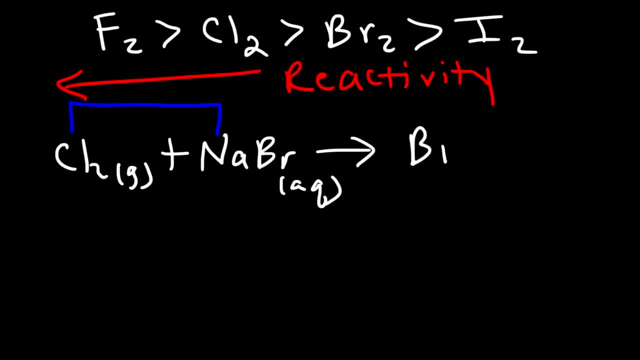 sodium. so we're going to get elemental bromine, which is in a liquid state at room temperature, and sodium is going to pair up with chlorine. now sodium has a positive one charge, chlorine has a negative one charge, so the charges are balanced in the one-to-one ratio. 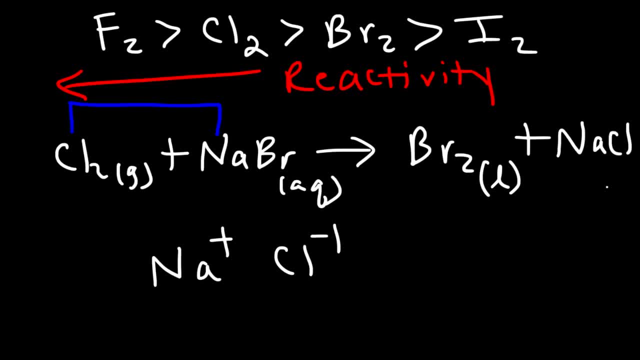 thus the chemical formula is simply NaCl and that is soluble. so we're going to write AQ to balance the chemical equation. all we need to do is put a 2 in front of NaCl and in front of NaBr and it's going to be balanced. 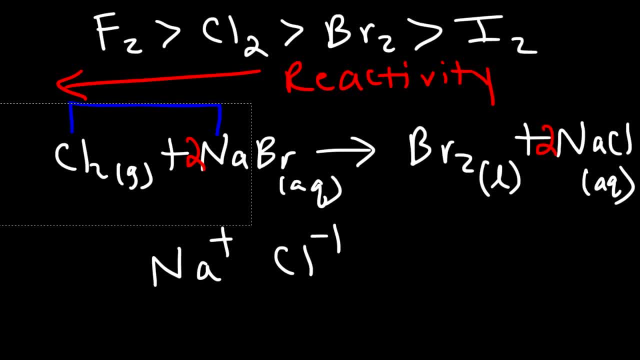 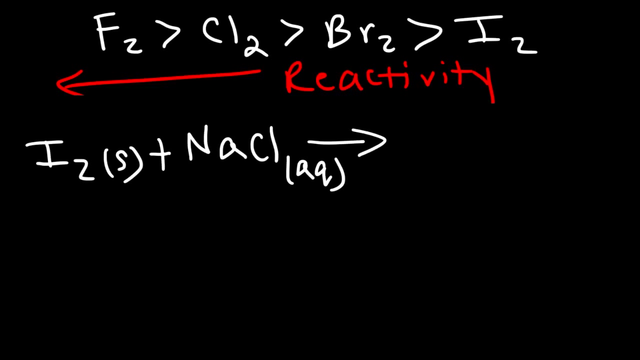 now I'm going to one more example, the final one for this video. so let's react solid iodine with aqueous sodium chloride. go ahead and predict the product of this reaction, or rather the products. so iodine, is it strong enough to displace the chloride? 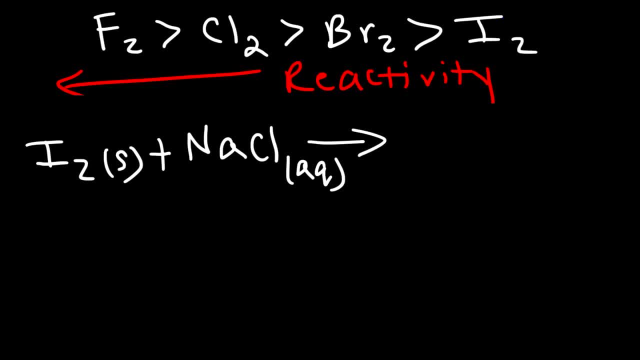 ion out of the solution. now, iodine is on the right side. it's less reactive than chlorine, so because it's weaker, this reaction will not proceed as written. so therefore, our answer is simply no reaction. iodine is not reactive enough to displace the chloride out of the solution. it's not going to work, and so